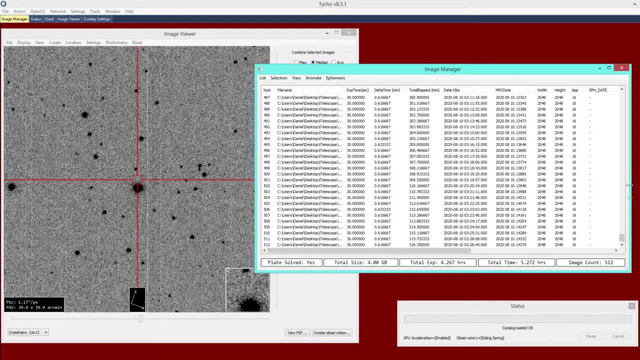 process. So what I have here is a sequence of 512 images, So each of these are 2k by 2k in resolution, 30 seconds in duration, And so what we've got here is basically it's similar to where you would do photometry of a minor planet, So you essentially capture a series of images. 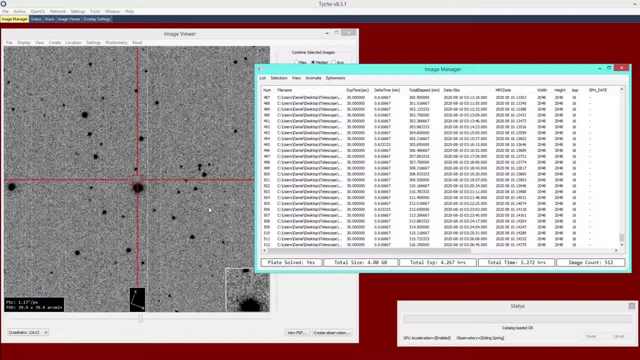 within this field of view. The object is present on every single image and you're going to compute the magnitude of that object over time and then hopefully be able to analyze that time period and essentially compute a period of time. So the difference is that with the variable star it's actually easier because it is stationary. 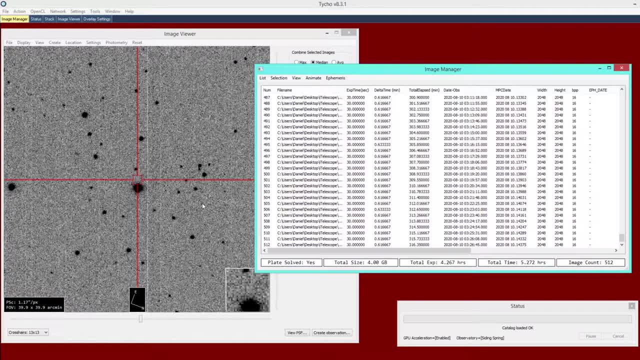 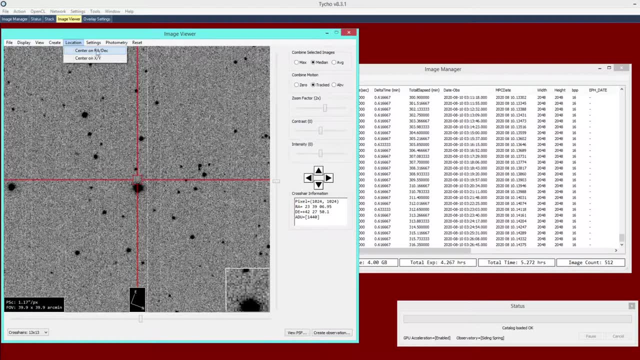 So, with this example here, I've gone ahead and loaded up these images into the image viewer And what we can do is go ahead and navigate to the location of the star. So go to location and if you know the right ascension and declination, then you can type in those coordinates here. 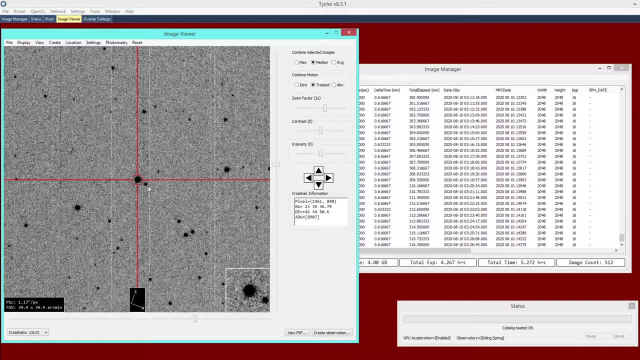 So I'm going to click OK. So here is the variable star And I'm going to go ahead and type in the coordinates here. So I'm going to click OK And, as before, you'll want to have a star catalog loaded that you're comfortable working with. 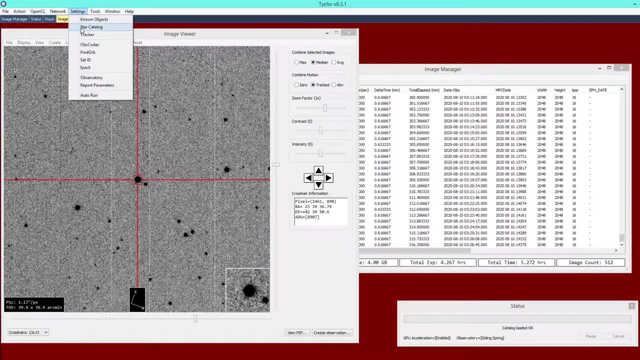 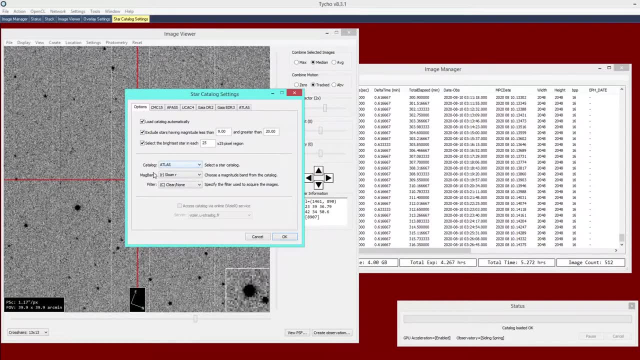 So for me I like to use the Atlas star catalog. It's very much ideal for photometry, And so this is the Atlas catalog, And I like to use the Sloan R magnitude band. That is the native magnitude band of this catalog. So I'm going to click, OK. 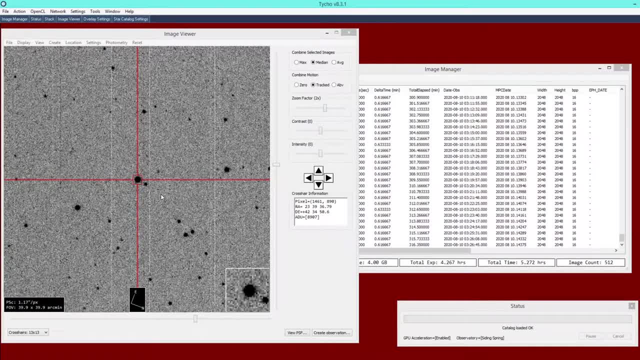 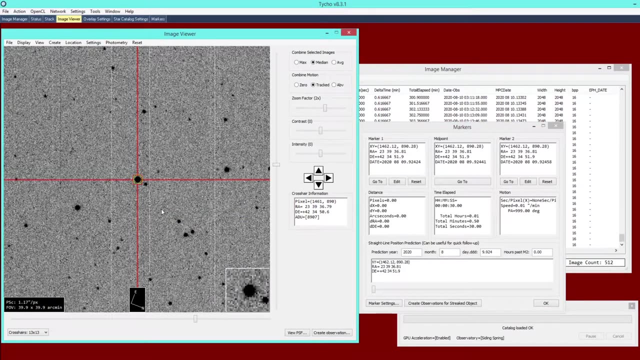 And what we can do is, as if it were a minor planet, we can go ahead and define two markers, Two positions, But in this case those markers will be identical. So it's stationary in position. So we create marker one, And then I create marker two. 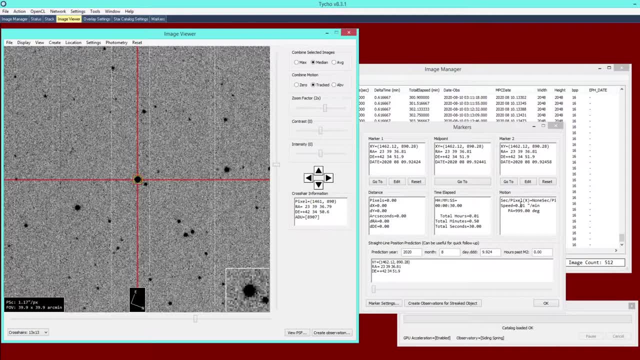 And, that being the case, there's really no motion. So it has a speed essentially of zero arc seconds per minute And the position angle is irrelevant. So we just go ahead and create a photometry set Using that information. Now, as I have mentioned in the other tutorial videos, 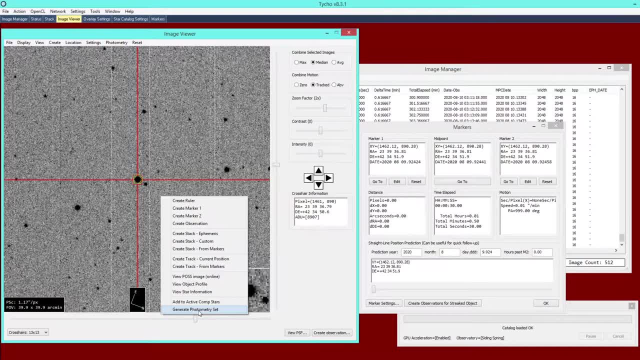 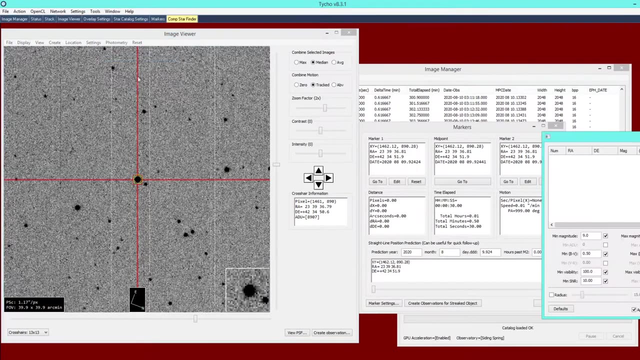 if you do not specify any comparison stars, then Tycho will assume that you want to use automatic comparison stars. So before I generate photometry, I am going to go ahead and manually define comparison stars. You can go to find comp stars from the photometry menu. 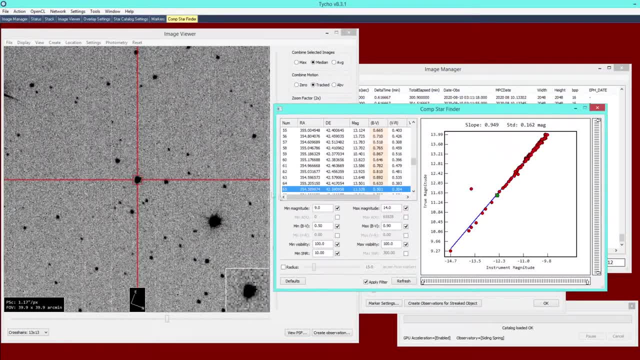 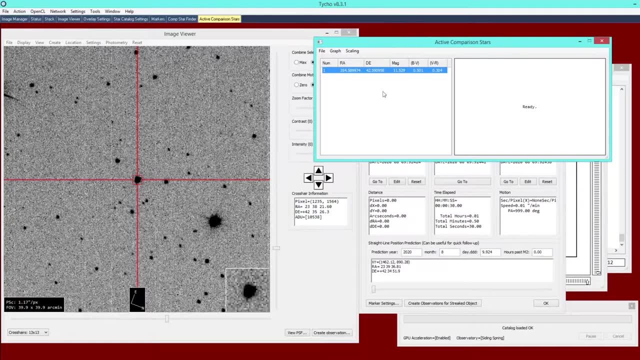 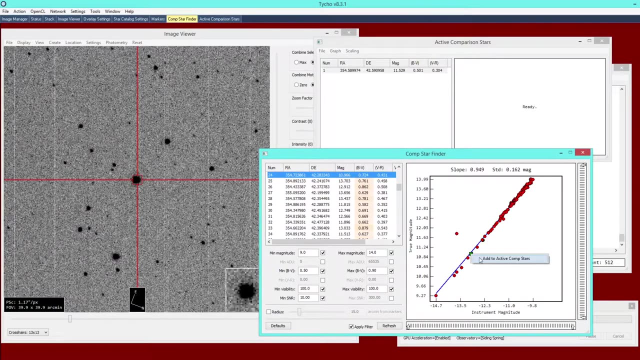 And this will present a new window here And you can choose your own comparison stars. So I might. if I want to, I can generate this list of active comparison stars Again using this comp star finder module. So if I want to just go ahead and populate this list with what appear to be reasonable, 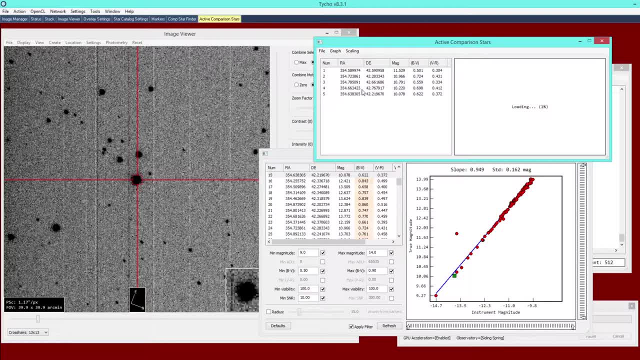 comp stars. I can go ahead and do that. So I've generated up a list of five comparison stars And what I'm doing right now is simply generating data on each of these comp stars And that's going to tell me whether or not they. 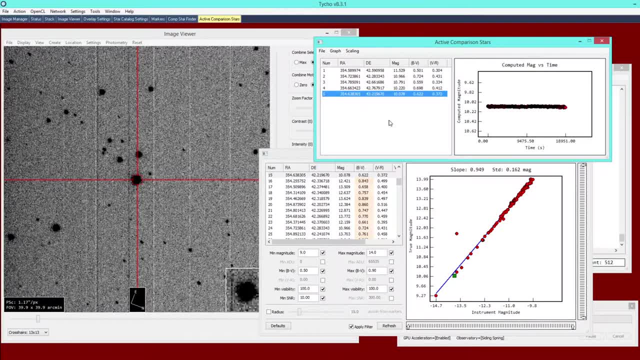 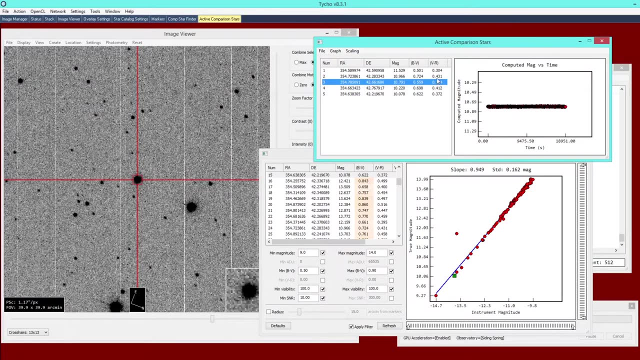 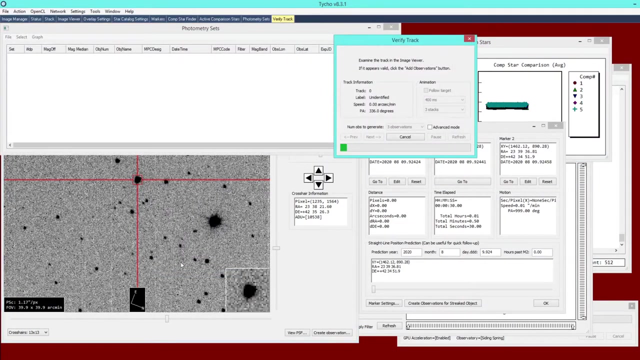 are quality comparison stars. Okay, so this appears to be a pretty good comparison star. It has a flat line here, So computed mag over time is consistent, And this is the same with all these other comparison stars. So again we can go to generate photometry set. 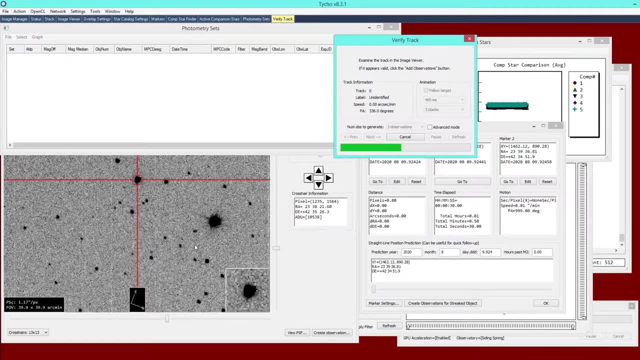 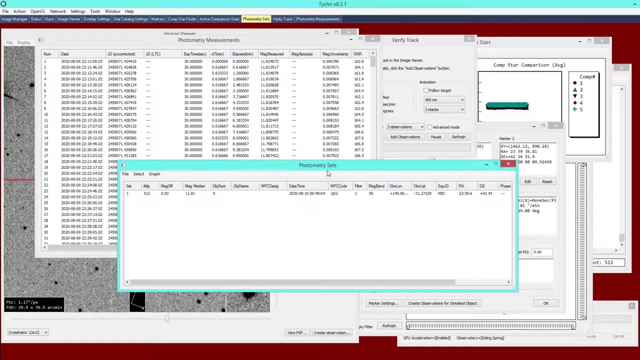 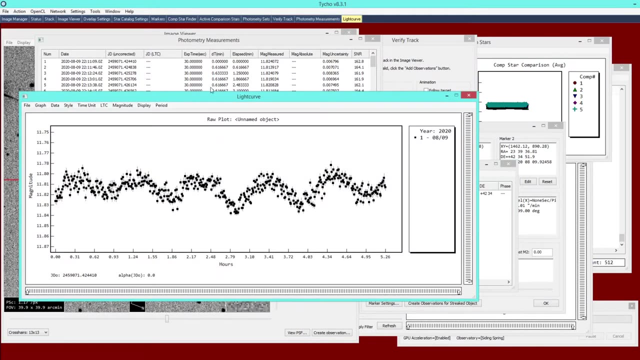 And that's going to using those two markers. it is going to generate magnitude measurements Of this object. So we now have one photometry set defined And I can go to graph plot all sets. So we only have one photometry set. so that's okay. 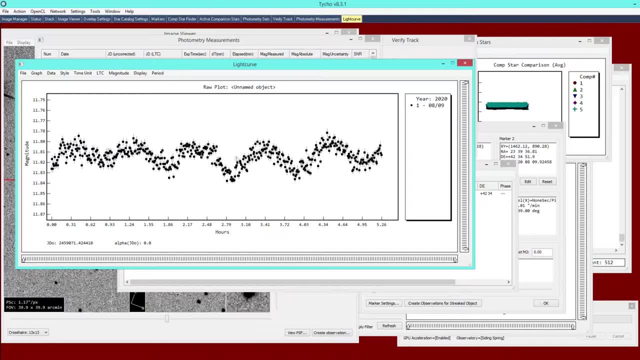 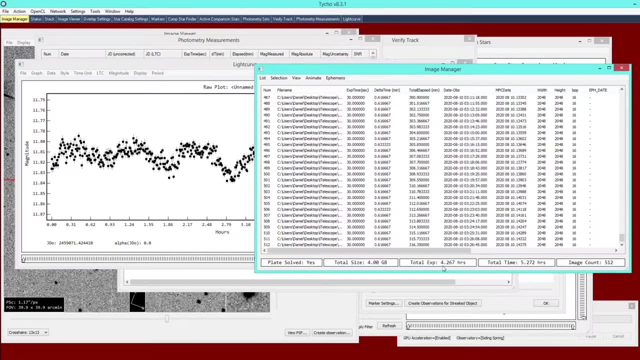 And what you can see here is the magnitude over time. So this is over. let's go ahead and take a look. This is over a four hour total exposure time period. The total time is 5.27 hours. So that would be. 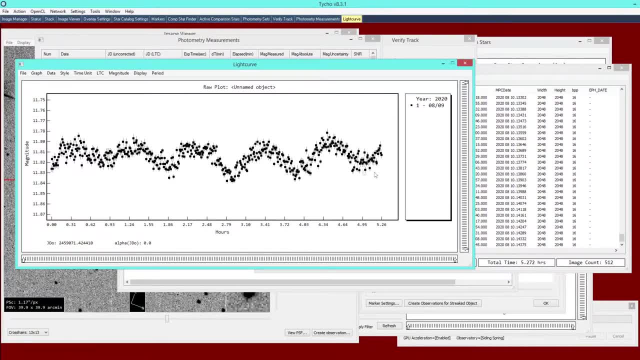 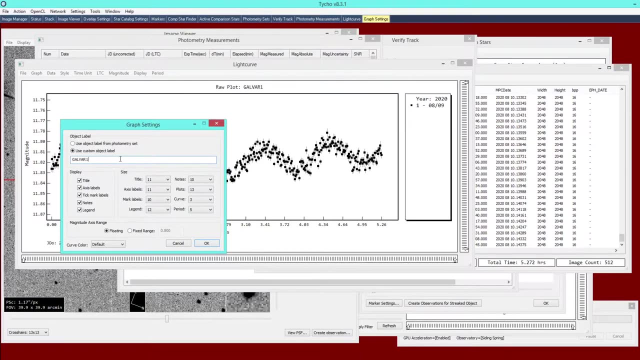 The actual time span from start to finish is 5.27 hours. So at this point, if we wanted to, we could try to. well, first we might want to go ahead and give it a label. So if you want to, you can type in Galvar 1 or whatever the name of your object is. 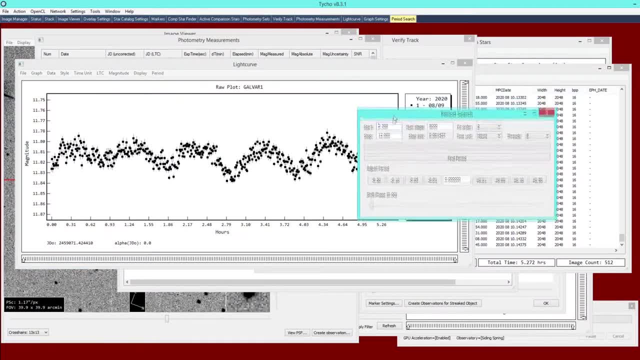 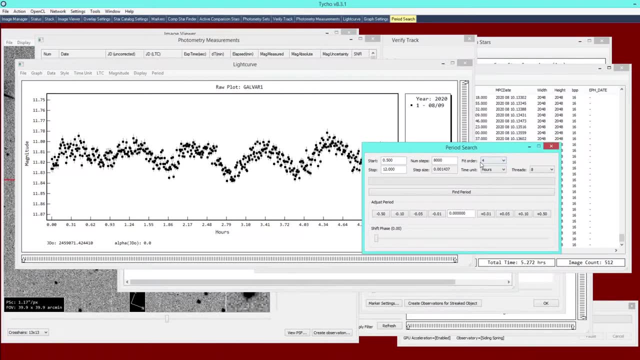 And I can go ahead and click find period. And in this case, because this is not a minor planet, we want the fit order to be different. So normally you would choose four as the starting fit order. for a minor planet, You might even use a higher order. 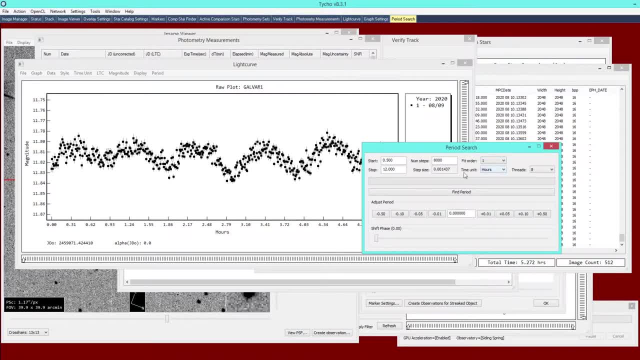 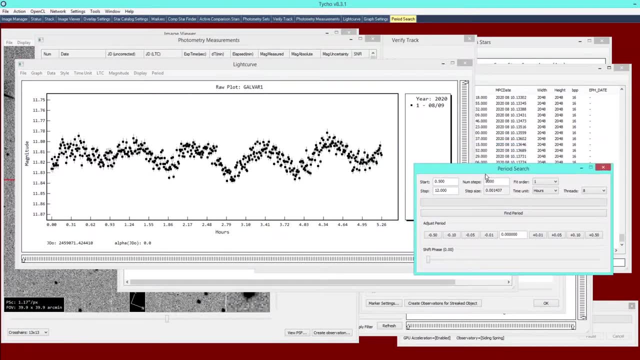 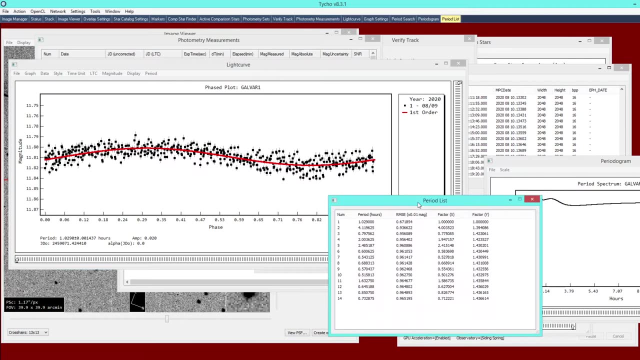 But for this example I'm just going to use a fit order of one, because we're not searching for a bimodal curve. We're actually just looking for the period from one peak to valley. So I click find period And what we have here is a list of candidate periods. 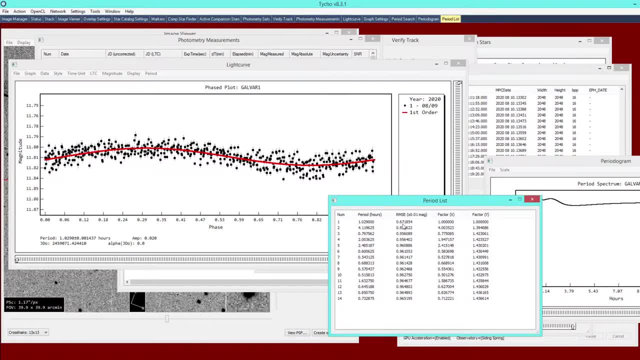 And it says that the first candidate period here is 1.029 hours. Now I might want this to be in minutes, So I can go ahead and switch the time unit to minutes, And now you'll see this update here. So it says 61.74 minutes. 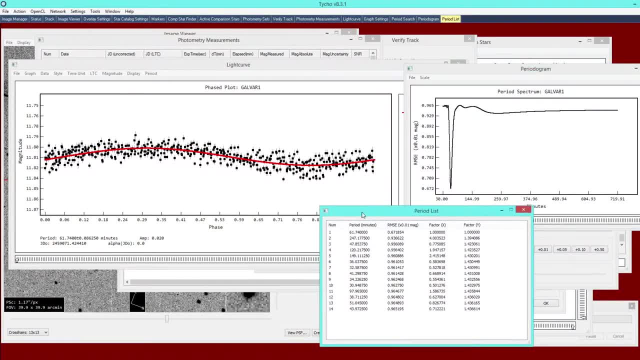 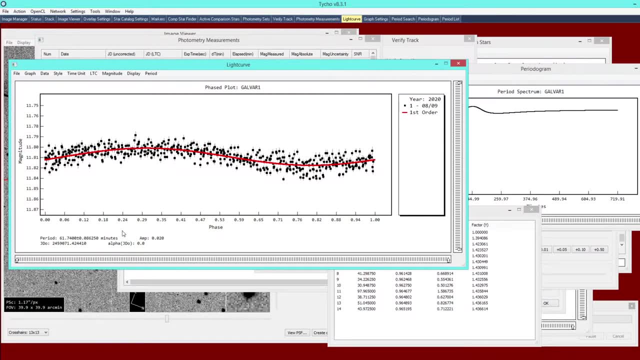 And here's the period spectrum So you can get an idea of what that looks like. But again, this is a fit order of one. So first order fit, And, And our period here is 61.74 minutes And that actually compares quite favorably with the submitted period of this variable. 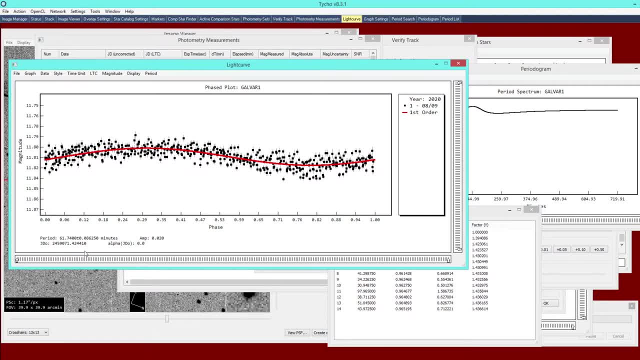 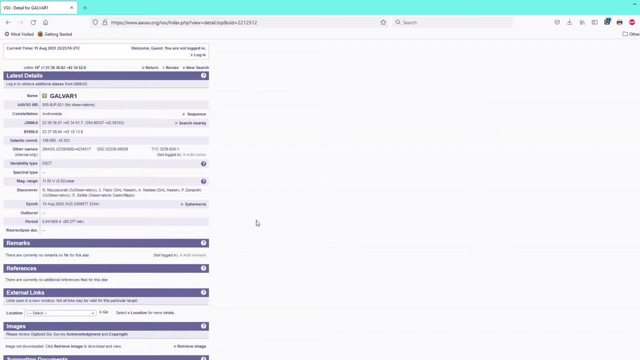 star. So if you wanted to, you could go to the AAVSO website And I brought up the information on this variable star. So galvar1 is the name And the published period is 60.277 minutes And, as it turns out, that's well within the expected. uncertainty, if you will, of this. 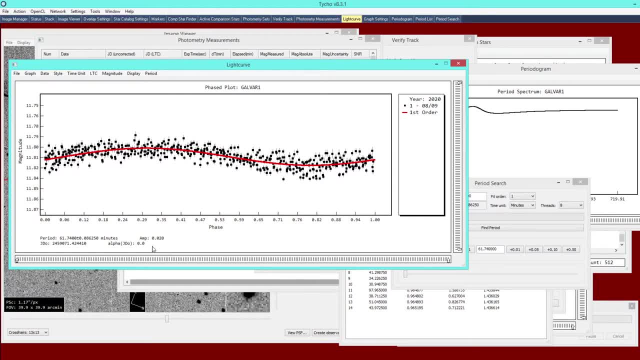 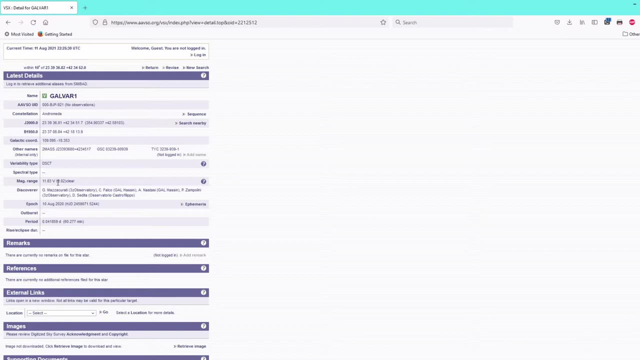 particular object And the amplitude determined by Tycho. it computes it as being 0.02 magnitudes. So if we compare that again with the published result here we have magnitude range 11.83.. And the amplitude, if you will, of 0.02.. 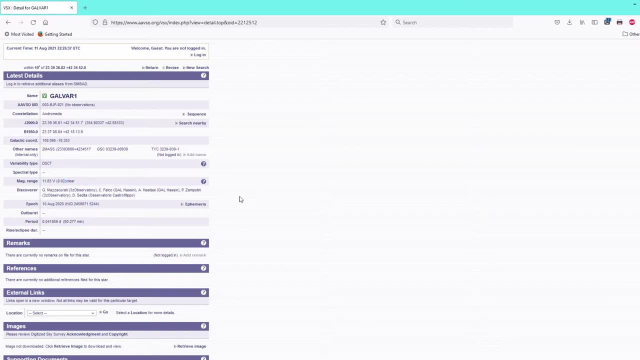 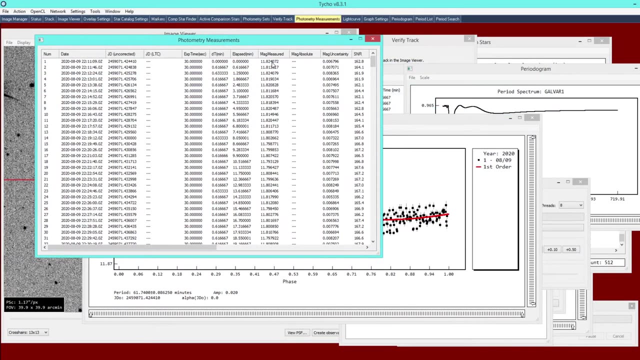 So 0.02.. Again, Again With the computation done by Tycho, And 11.83.. And if I look at the photometry measurements, 11.83 is well within the range of photometry measurements that we have here.